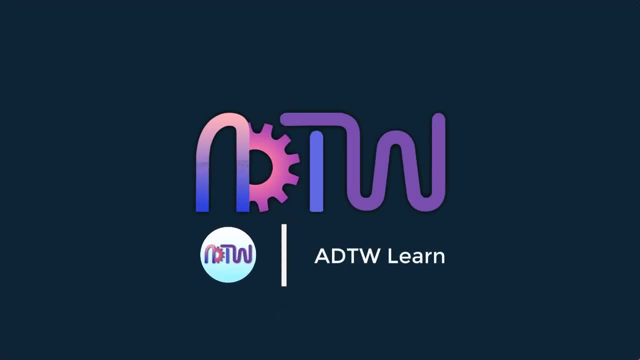 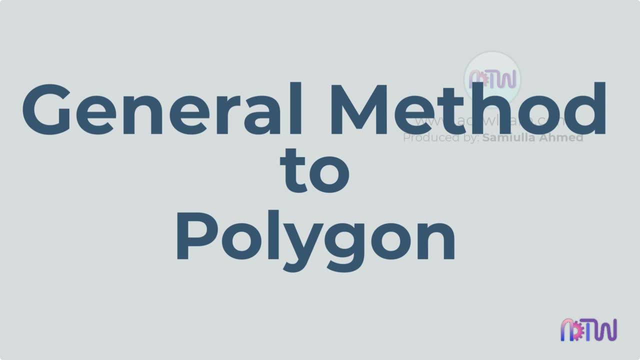 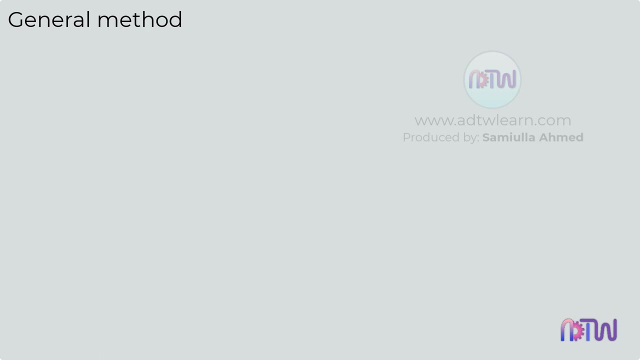 In this video, we will learn a general method to draw any polygon. To draw any polygon, draw a line whose length is equal to the required side length of the polygons. In this video, I will draw a line of 50 mm in length. Remember this length. 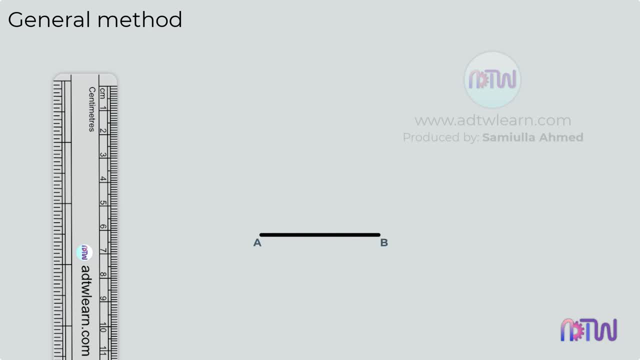 can be anything. Label the endpoints as A and B. After this, draw a perpendicular line at point B and the length of this line should be the same as the horizontal line, That is, 50 mm. in this case. Name this endpoint as point C. Take a compass. adjust the compass. 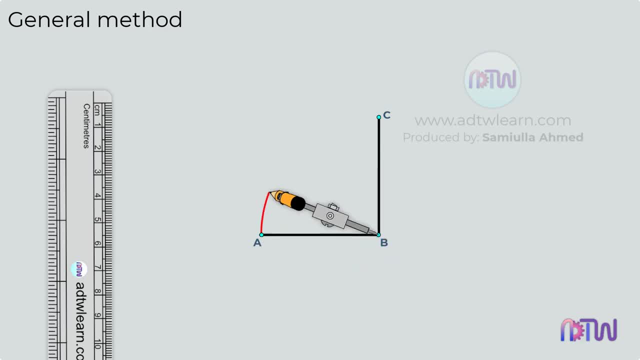 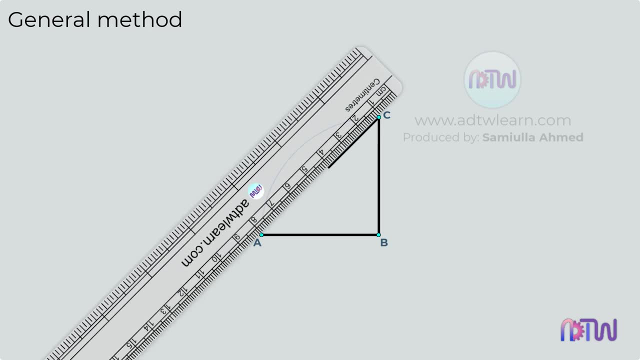 to length AB and, using point B as a center, draw an arc from point A to point C. Next, take a ruler and draw a line joining point A and C. After this, we need to divide this length AB into two equal parts. 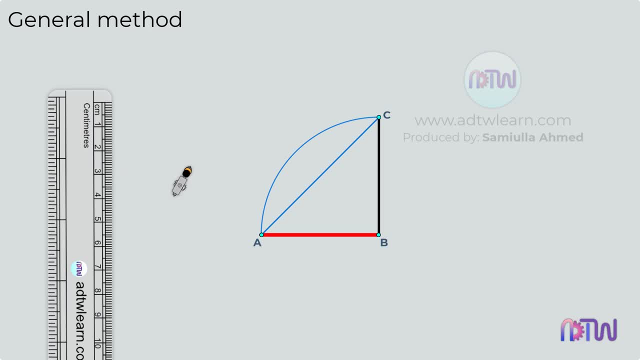 To do so, we will apply the middle point method. Take a compass, take some length on the compass and use points A and D as centers. cut arcs above and below this horizontal line. Draw a line passing through these points. Label these points as 4 and 6.. After this we need: 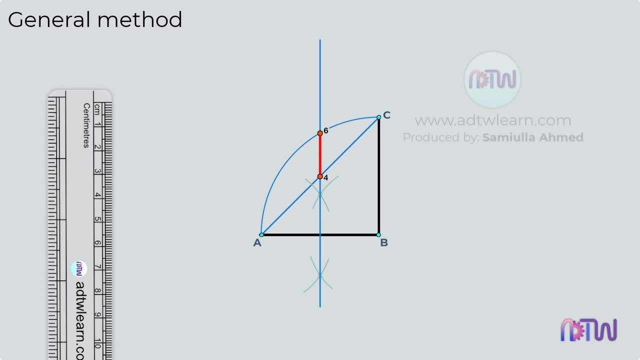 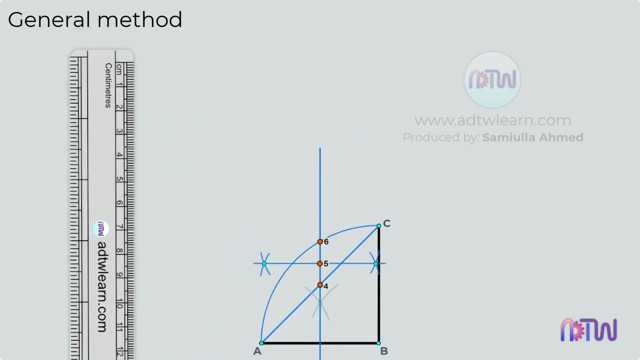 to divide this length between points 4 and 6. and 6 into 2 halves. To do so, apply the middle point method. Draw a line passing through these points and label this point as 5.. After this, take a compass and adjust it to this length between points 5 and 6, and cut. 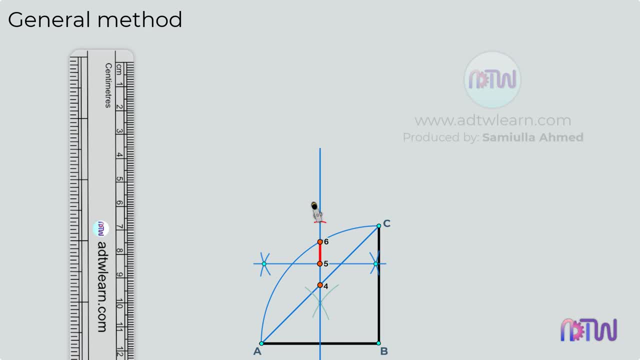 arcs on the vertical line. Name these points as 7,, 8, and 9.. Therefore, we got the center points of all the polygons. If we draw a circle using the length between point 4 and a, we will get a square. 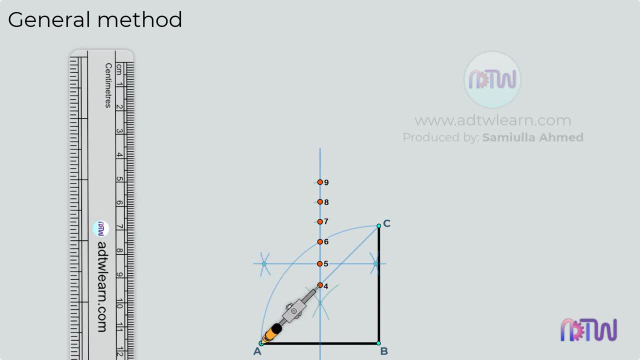 Adjust the compass to the length between 4 and a and draw a circle using point 4 as a center. Next, take the length of side a- b on the compass and cut arcs on the circumference of this circle and join these points with a line. 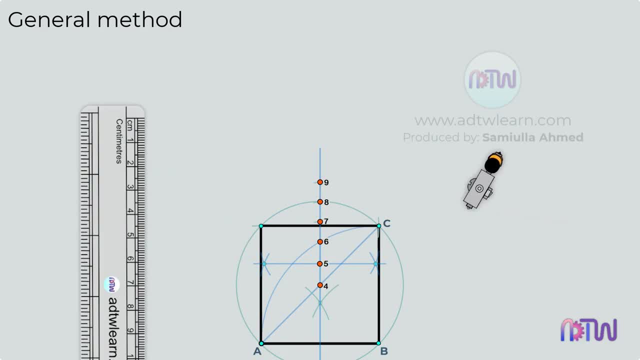 This will result in the square. Next to draw a pentagon, adjust the compass to the length between point 5 and a and, using point 5 as the center, draw a circle. Adjust the compass to length a- b and use this length to cut arcs on the circumference. 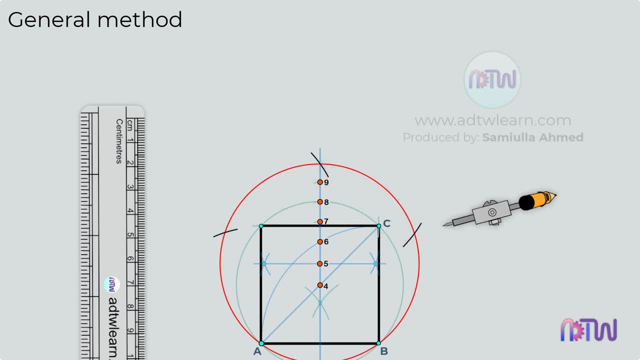 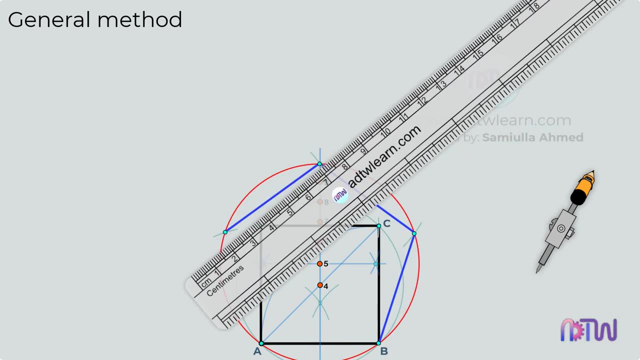 of this circle. So today we cut, deal and draw the circumference of this circle. Use the compass and cross- IQ ruler to calculate the length of each white circle. If we join these points, we will get a pentagon. Similarly we can draw other polygons. 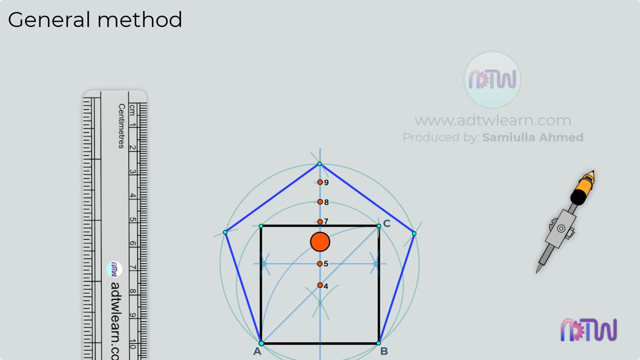 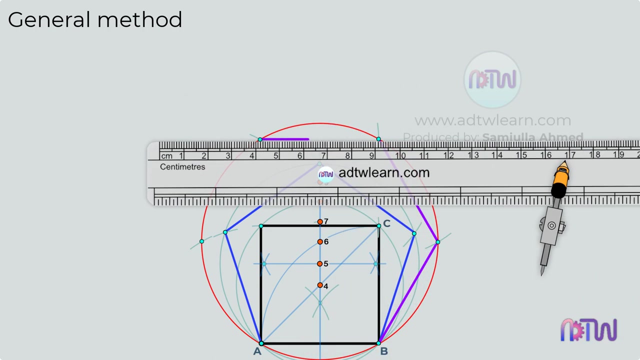 To draw a hexagon, adjust the compass to the length between point 6 and a and, using point 6 as the center, draw a circle. Adjust the compass to length b and use this length to cut arcs on the circumference of the circle. If we join these points, we will get a hexagon. 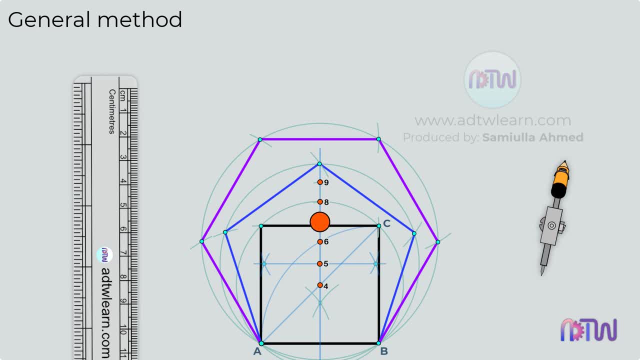 To draw a heptagon. adjust the compass to the length between point 7 and A and, using point 7 as the center, draw a circle. Adjust the compass to length AB and use this length to cut arcs on the circumference of. 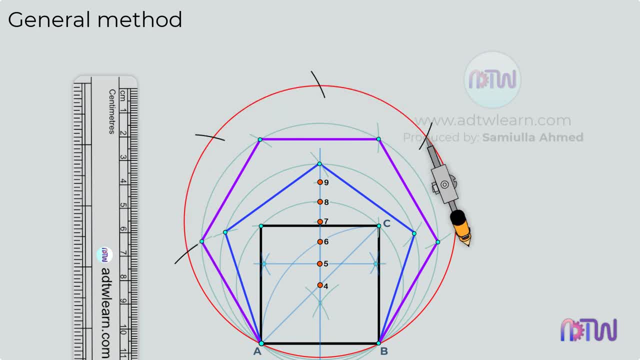 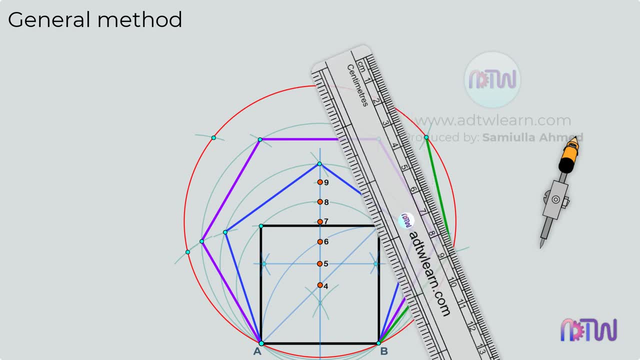 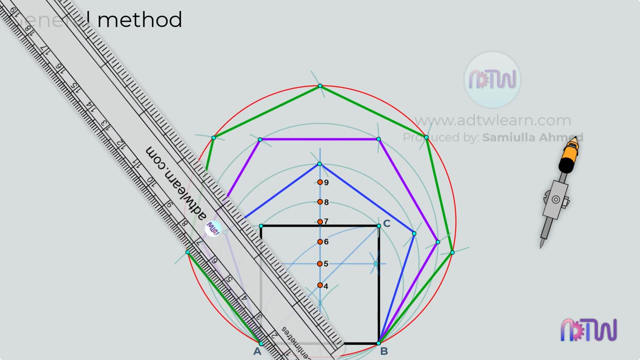 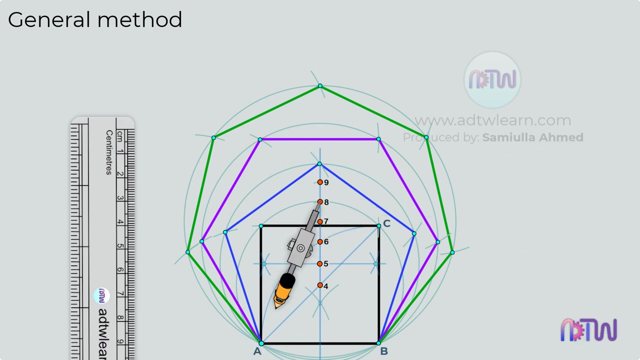 the circle. If we join these points, we will get a heptagon. To draw an octagon, adjust the compass to the length between point 8 and A and, using point 7 as the center, draw a circle. Adjust the compass to length AB and use this length to cut arcs on the circumference of.